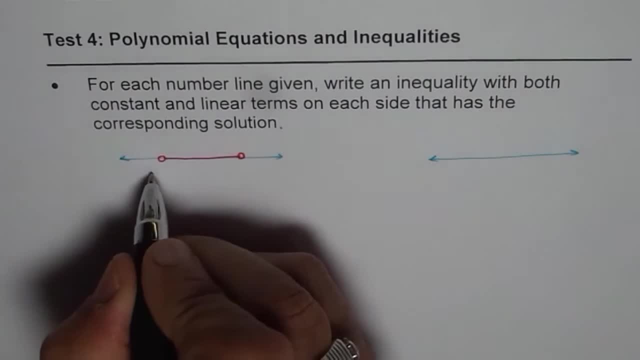 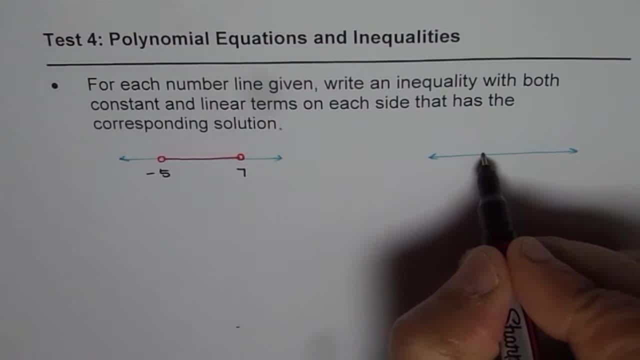 which is kind of like this: and these intervals are, let us say, minus 5 and 7 for us. On the other line, what I will take is I will take solid value that is filled in circle and one side. Okay. So let us say this value is minus 2 for us and it goes forever. Now you need 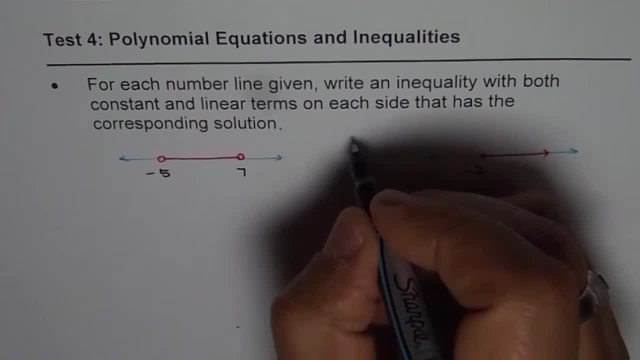 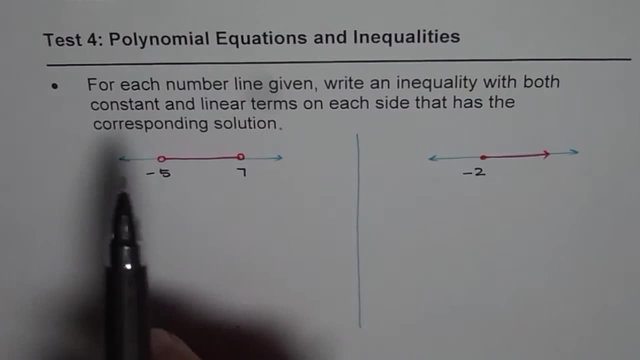 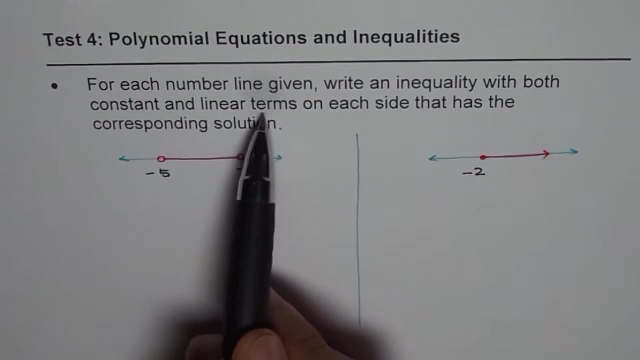 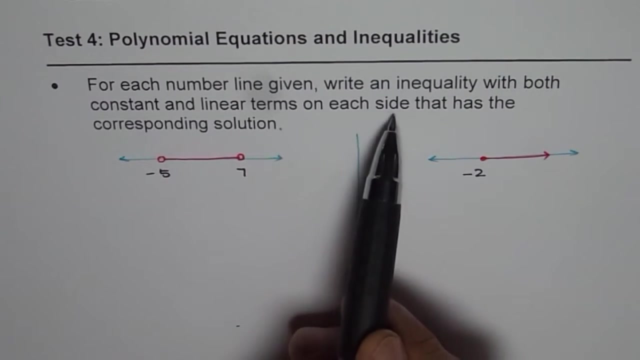 to write two inequalities, rather double inequalities, as the question suggests, right. So since we have a solution like this, right For each number line, write an inequality with both constant and linear terms. So we should have terms which are both constant and linear on each side. that has the corresponding solution. Now, on this number line, the solution is that: 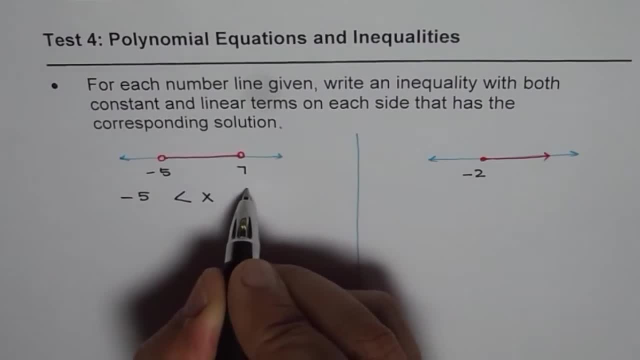 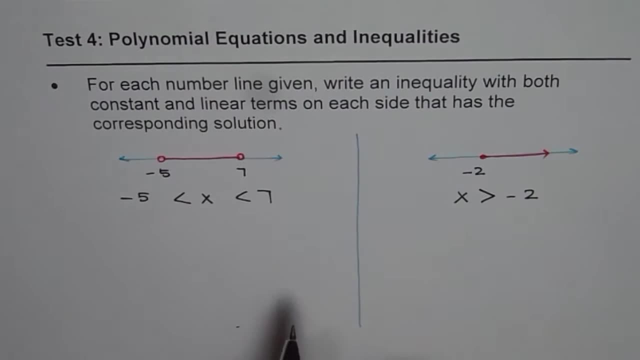 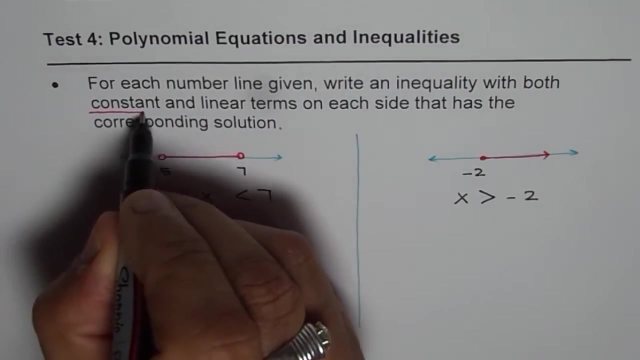 x should be greater than minus 5 and should be less than 7.. On this, the solution is that x is greater than minus 2.. So on both sides, we want both constant as well as linear terms. Right, That's a constant and linear terms. That means kind of like this: So we have two. 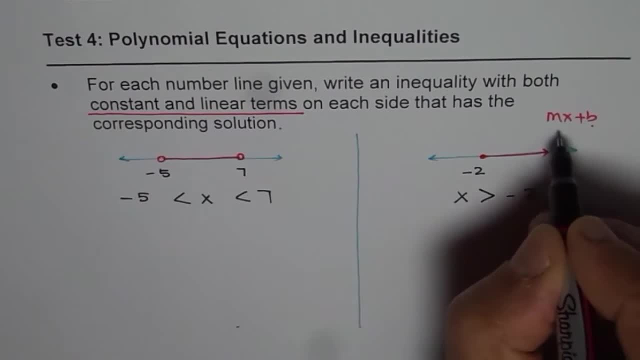 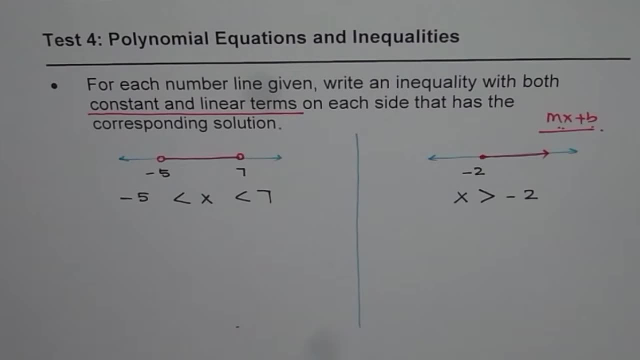 kinds of. you know mx plus b, right, So that's a constant and this is a linear term. I hope you get an idea right Now. don't make a mistake of just putting a constant or just putting a linear term. Okay Now, it's a very easy way to do it and that is why I am here to 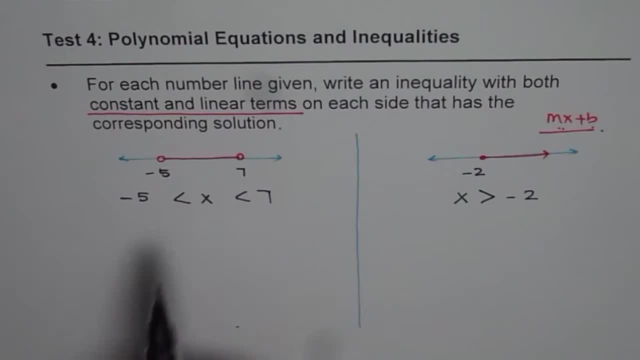 give you a good and a quick solution. So you need something like that on each side. So what we will do is very simple. Let us add some linear term. For example, we could add x plus 1 on each side. right, Maybe x plus 4? how does it matter? So if I add x plus 4 on each side, what do I get? That is: 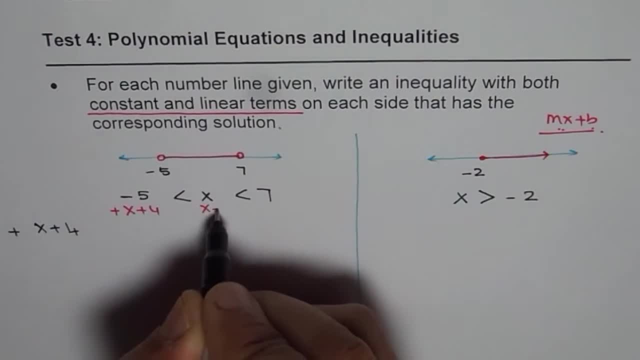 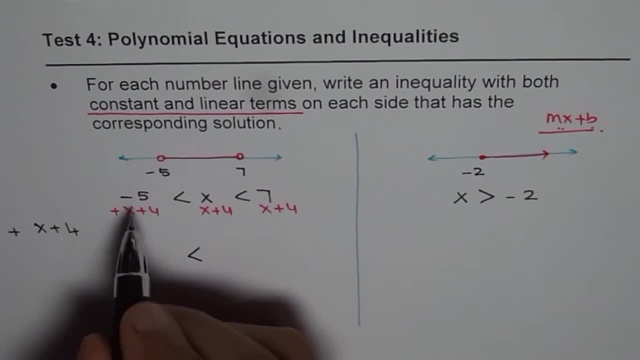 to say: I am adding x plus 4 here, I am adding x plus 4 here and I am adding x plus 4 here. The result of this is we get here x and 4.. 4 minus 5 is minus 1.. So we get x minus 1.. In this side we get 2x plus 4, which should: